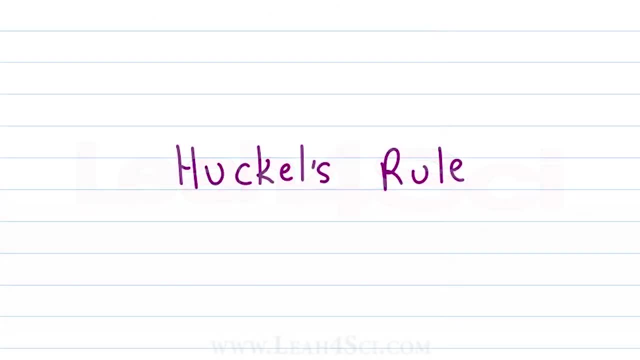 Leah here from leah4scicom, and in this video we're going to look at Huckel's rule in detail, followed by a shortcut to save you time when working out aromaticity problems. In the last video we looked at conditions for aromaticity where a molecule has to be cyclic. 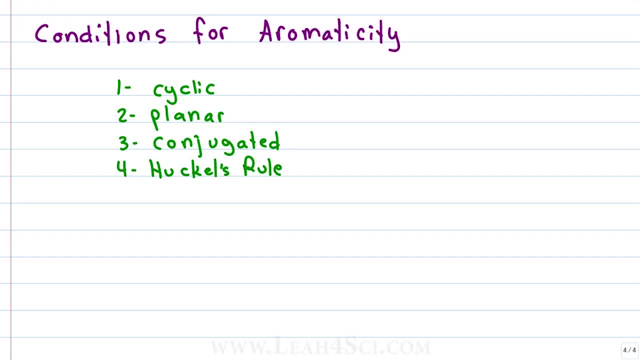 planar conjugated and follow Huckel's rule to be qualified as aromatic. The first three can be identified just by looking at the molecule, but Huckel's rule required solving for the equation 4n plus 2 is equal to pi electrons. When you're under pressure of an exam, you don't have that. 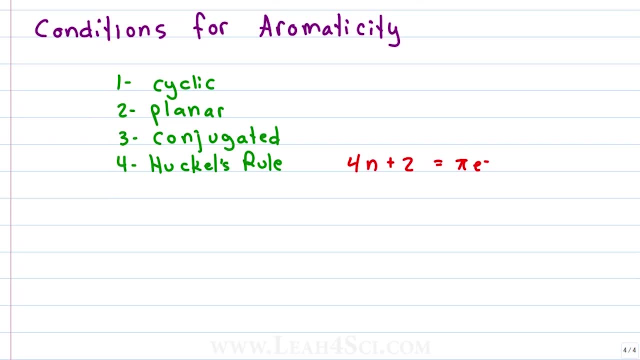 kind of time. You ideally want something fast that you understand. so you're confident with your answer and able to move on to the next question. If we analyze these two molecules using the conditions for aromaticity, we'll notice that they're both rings the first and last carbon. 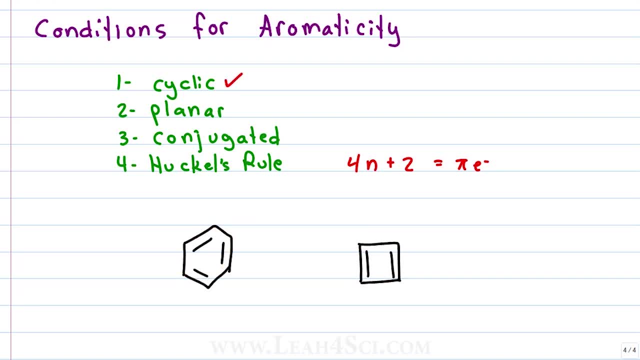 are attached to each other. They're both planar, since every carbon has a pi bond. every carbon is sp2 and every carbon is sp2.. So we can see that the first and last carbon are attached to each other. They're both planar, since every carbon has a pi bond. every carbon is sp2 and every carbon is sp2.. So we can see that they're both rings. the first and last carbon are attached to each other. We can see that they're both rings. the first and last carbon are attached to each other. We can see that they're both rings. the first and last carbon are attached to each other. They're both sp2 hybridized. 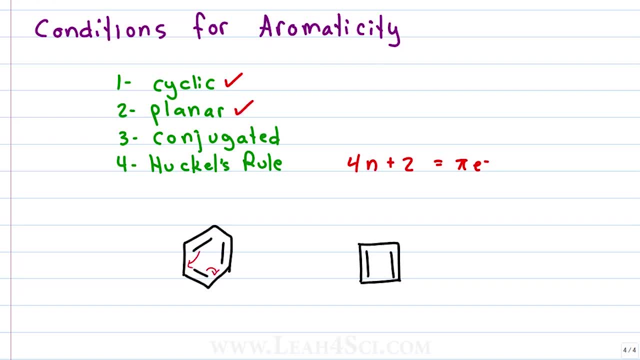 making the entire system planar. You can resonate around both of these rings, making both of these systems fully conjugated. But if you analyze the energy of these molecules, you'll notice that benzene is a very stable, not very reactive compound and cyclobutadiene is very unstable to 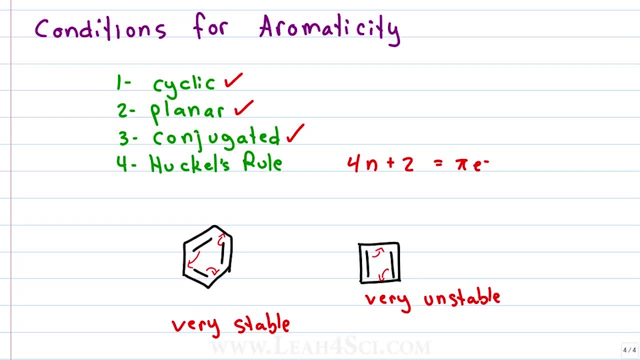 the point where it'll actually react with itself because it's so unhappy as it is. How do you figure this out out of the equation? I'm going to show you how to do it. I'm going to show you how to do it out of a laboratory setting. This is where we have to solve, for 4n plus 2 equals pi electrons. 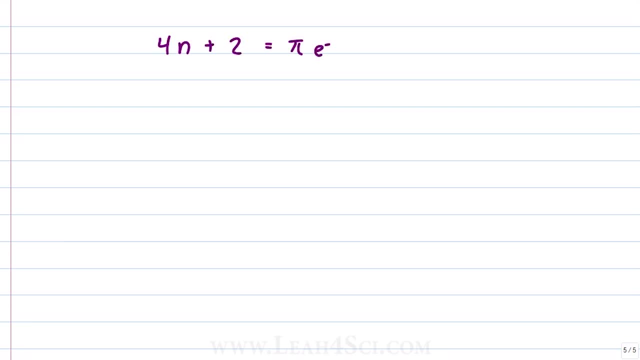 When we say 4n plus 2 equals pi electrons. this is a slight simplification. Most of the aromatic compounds you see will have the pi electrons, but you'll also see molecules that have lone electron pairs, that participate in resonance and are therefore part of the conjugated system. So 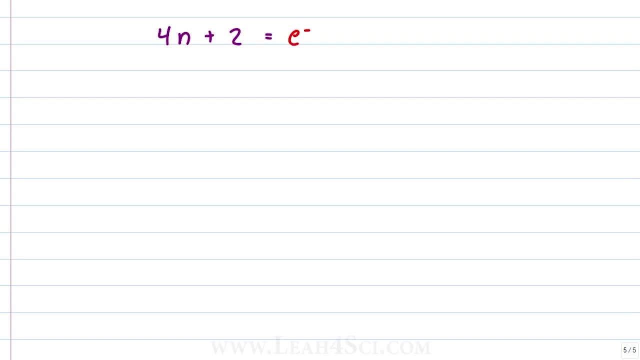 instead we should change this to say: 4n plus 2 is equal to: 4n plus 2 equals pi electrons. So to solve for 4n plus 2 equals pi electrons, we need to find the balance between pi electrons and 4n plus 2, which is equal to electrons, where we're specifically referring to all resonating. 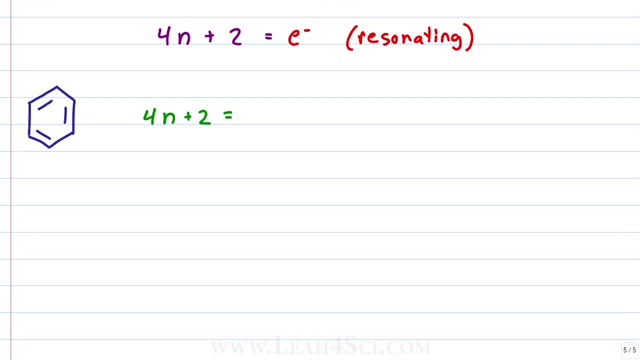 electrons. We'll start with benzene, since we're most familiar with it, and set up the equation 4n plus 2 is equal. Let's see 1,, 2,, 3,, 4, 5, 6.. We have six pi electrons, all capable of resonating. 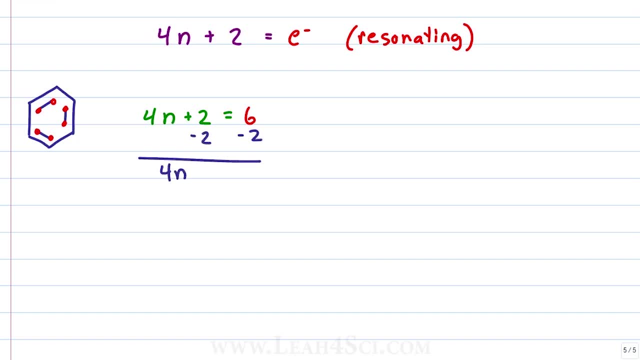 Let's solve for n. To solve for n, we subtract two from both sides, giving me 4n plus zero, or 4n plus zero n is equal to 6 minus 2, 4.. Then we divide both sides by 4 to isolate n. divide both. 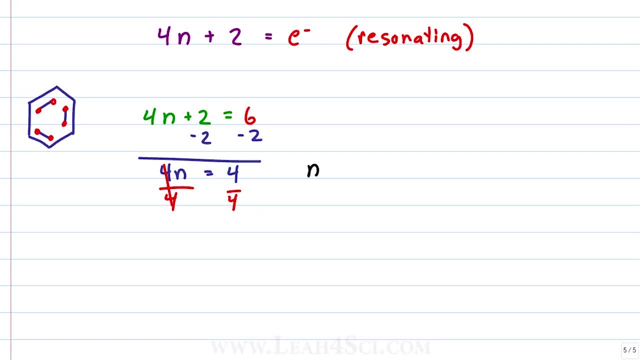 sides by 4, and this gives me: n is equal to 4 over 4, a number divided by itself is equal to 1, n equals 1.. What's the significance of 1? Nothing, except for the fact that it's a whole number. 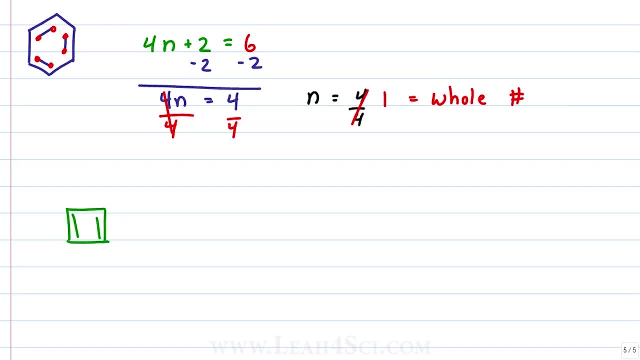 Now let's look at our other example of cyclobutadiene, which we already said is so unstable. it'll react with itself. Let's see how Huckel's rule justifies that By setting: 4n plus 2 is equal to 1,, 2,, 3,, 4, 4 pi electrons. Subtract 2 gives me 4n plus 0, or 4n is equal to 4 minus. 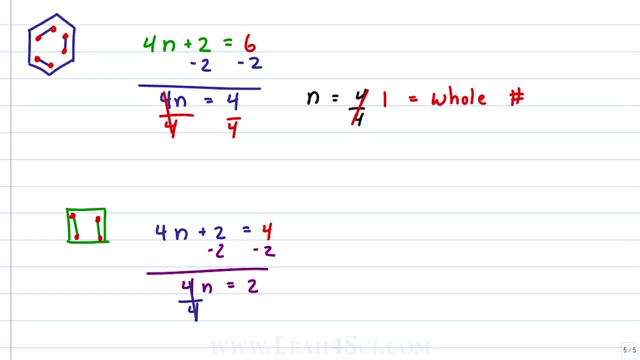 2 or 2.. Divide both sides by 4, which gives me n plus 2.. So we have: n is equal to 2 over 4, 2 over 4 can be reduced to 1 over 2.. It doesn't matter. 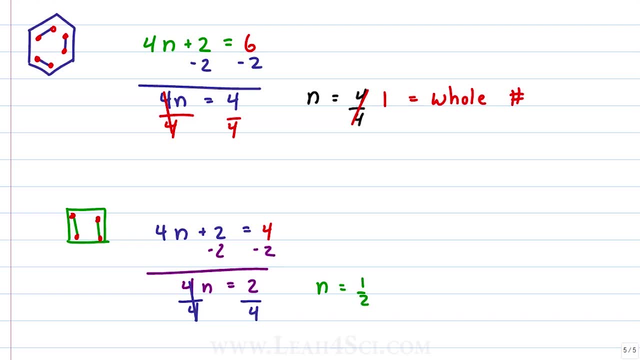 which one we use, because fact of the matter is 1 over 2 is a half, half is a fraction, and that means this disobeys Huckel's rule. This helps us understand why this molecule is so unstable and why it is not considered aromatic. 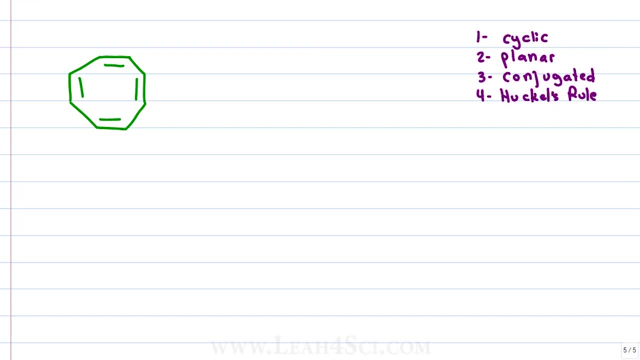 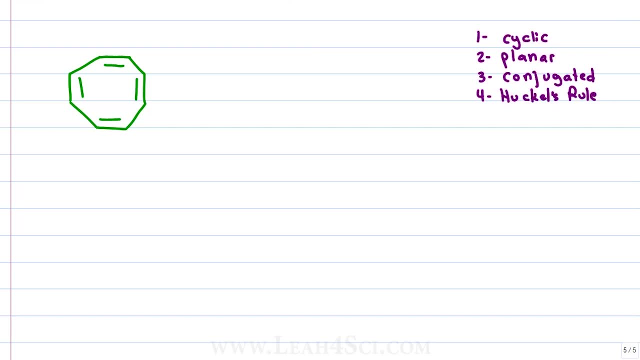 4, 0, 0, 0, 1, 0, 1, 0, 0.. We have a total of 8 carbons that appear to be in an aromatic ring. The molecule is cyclic. Carbon 1 and 8 are attached to each other. The molecule. 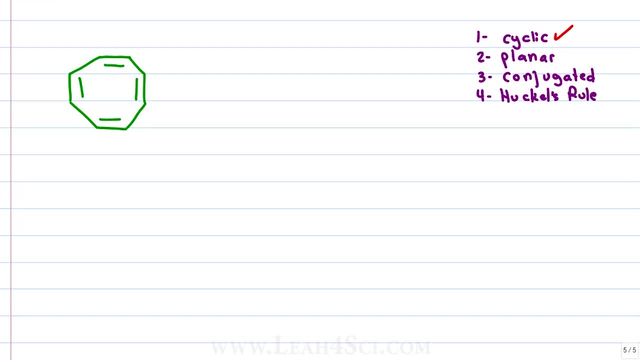 is all sp2, hybridized carbon atoms, with pi bonds all around the system. The way it's drawn right now, it appears to be planer. The pi bonds can resonate over the entire ring, making it's conjugated, but does it obey Huckel's rule? 4n plus 2 is equal to 8 pi. 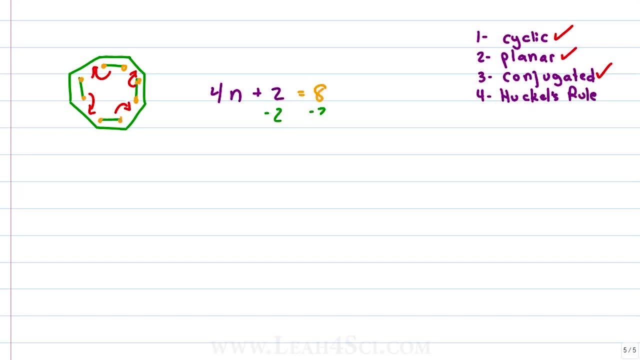 resonating electrons. solve for n subtract two on both sides, giving me 4n is equal to 6, divide both sides by 4, which gives me n is equal to 6 over 4, you can simplify this to 3 over 2 or 1 and a half, doesn't matter, it's not a whole number, it's a fraction. and 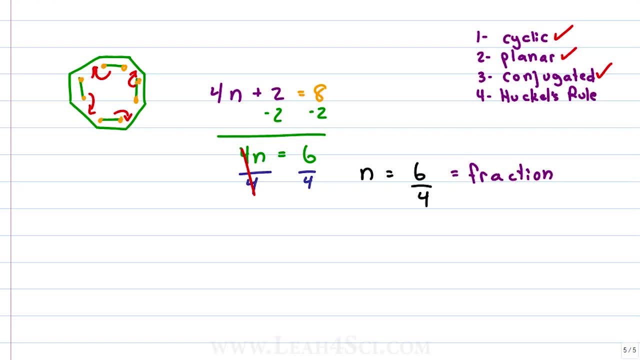 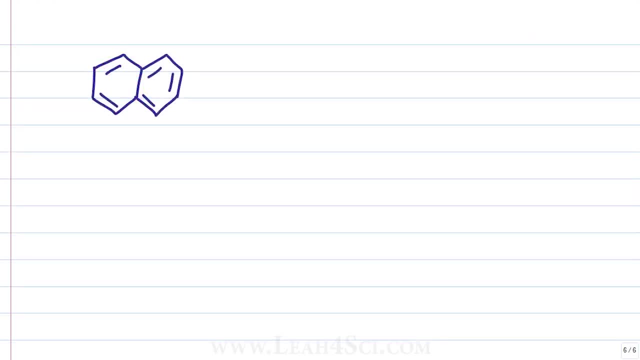 that means this molecule disobeys Huckel's rule, is unstable and not considered aromatic. Take a look at this interesting system. we have not one but two rings, recognizing that resonance can go outside of the first ring, making the entire system conjugated. that 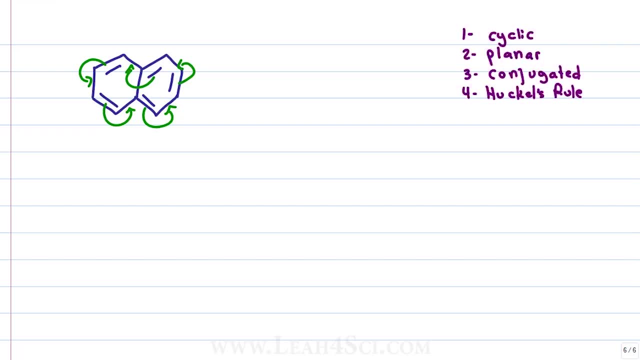 means it's potentially aromatic. let's see. Is it cyclic? Yes, It's a bicyclo compound, but that still qualifies as cyclic. All the carbons are sp2, we have pi bonds everywhere. that makes it planar. We've shown that it can resonate over the entire system, making it conjugated and when. 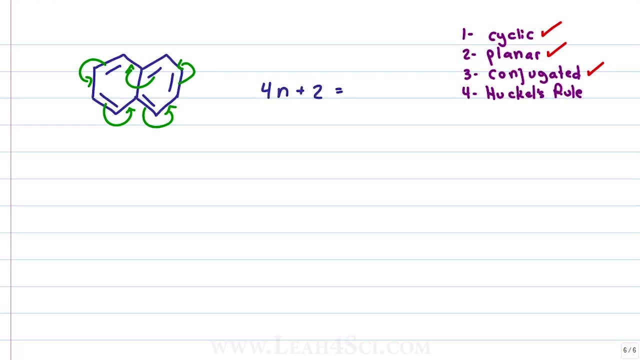 we apply Huckel's rule. we apply it to the entire resonating system, which means we set 4n plus 2 equals 10 electrons. If we solve for n, we subtract two on both sides, which gives us 4n is equal to 8, divide. 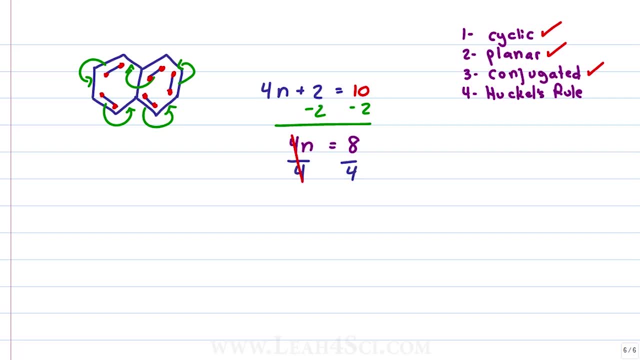 both sides by 4, cancels out the 4 and gives us that n is equal to 8 over 4, which can be simplified to 2 over 1.. No, this isn't a fraction, because any number over 1 is that number. it's a whole number. 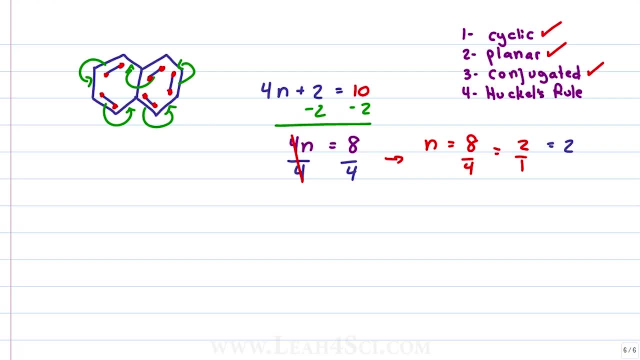 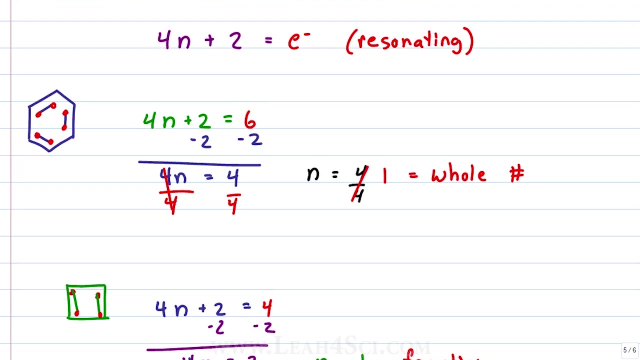 in this case 2.. That means a 10 electron system does obey Huckel's rule and is aromatic. Why did we go through all of these problems? Let's go back to all of this again. When we had 6 electrons, we got a whole number. it was aromatic. 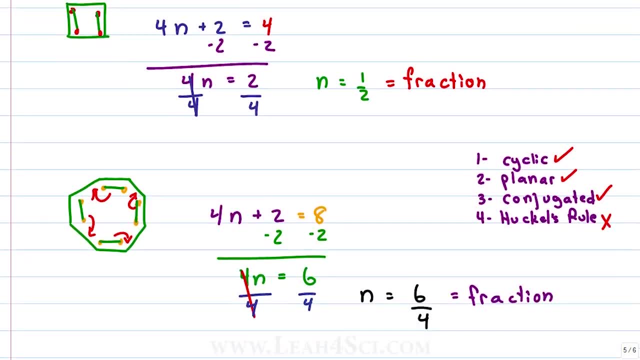 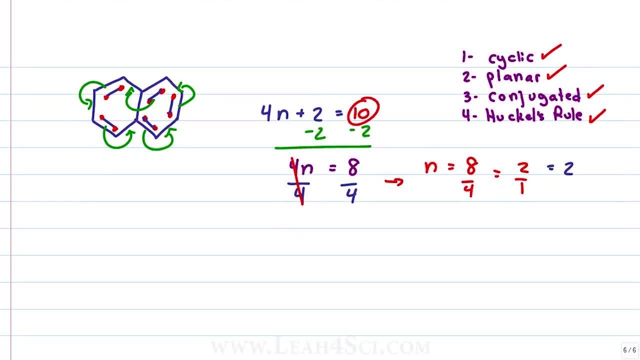 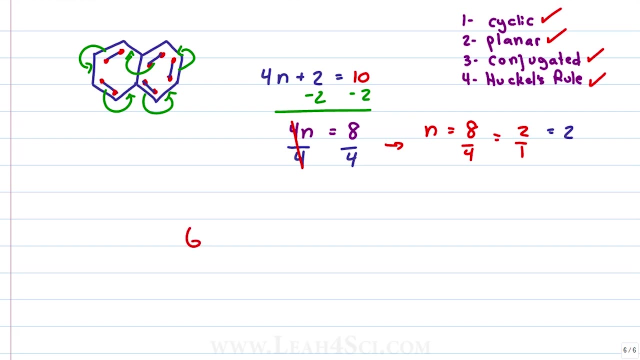 Four electrons- not a whole number, anti-aromatic. Eight electrons- also fraction- anti-aromatic. Ten electrons, whole number aromatic. What if we write these out as a pattern? We know that 6 is aromatic, we know that 10 is aromatic, we know that both 4 and 8 were. 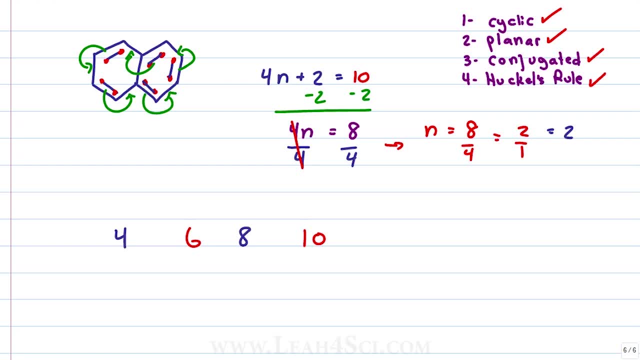 anti-aromatic. well, what if we continue? If you do the math, you'll notice that 2 gives you a whole number. then on the right, 12 is a fraction, 14 gives a whole number, 16 is a fraction, 18 is a whole number and the 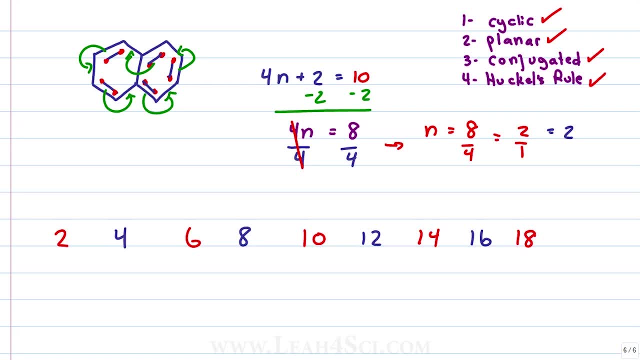 pattern continues. Don't take my word for it. prove it to yourself by solving: 4n plus 2 equals all of these numbers. This specifically refers to the number of electrons. This specifically refers to the number of electrons In organic chemistry. the faster you get through a problem, the quicker you move on to the. 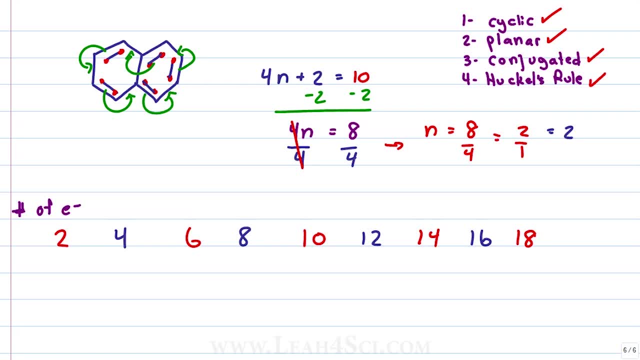 next one, the more likely you succeed on your exam. so let's make this even simpler. Unless we're dealing with radicals, electrons are always in a pair. We have electron pairs in a pi bond and we have lone electron pairs. So let's ask ourselves: if we have 2 electrons, how many electron pairs do we have? 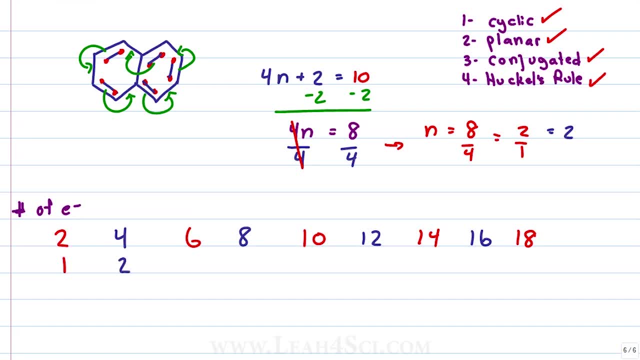 1. If we have 4 electrons, 2. 6 electrons, 3. And so on. This is how you can identify Huckels rule without working through the math. First, determine if your molecule is cyclic, planar and conjugated. 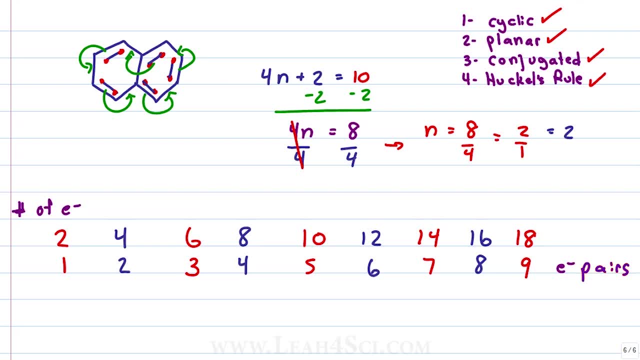 If yes, count the resonating electron pairs and ask yourself: do I have an odd number of electron pairs? If yes, this molecule obeys Huckels rule. Do I have an even number of electron pairs? If yes, this molecule does not. 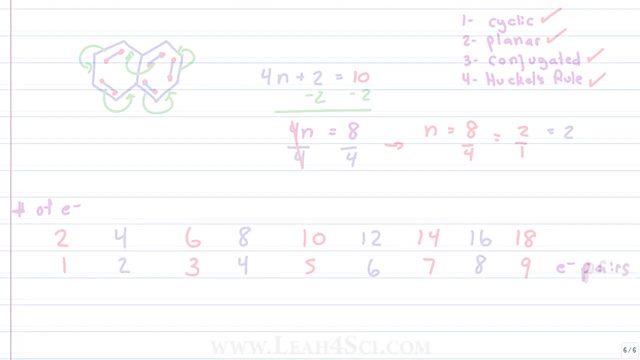 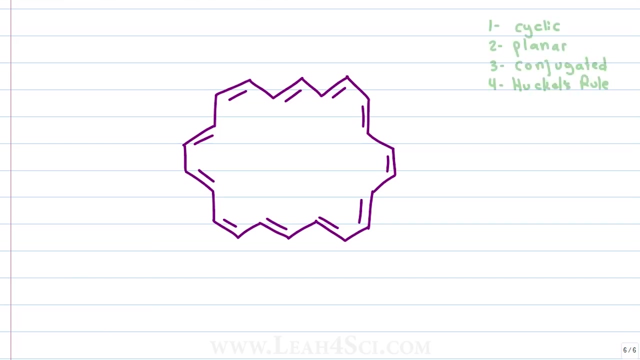 obey Huckel's rule. For example, let's say I showed you this molecule and asked you to determine if it was aromatic or not. Looks a little scary, but let's break it down. This is why it helps to have a system to follow so that, no matter how terrifying it is, you 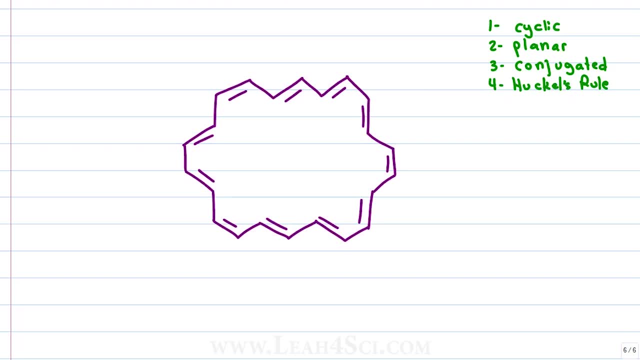 know exactly what to do. Is this molecule cyclic? Can I trace a path around the entire molecule so that the first carbon attaches to the last carbon? Absolutely yes. Is this molecule planar, Without building it on a model kit? recognize that every single carbon atom has one pi bond. 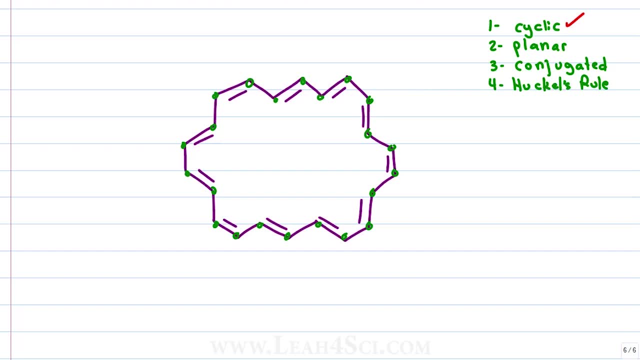 no charges. that means they're sp2 hybridized, and if they're all sp2 hybridized, the molecule is planar. Next we look for conjugation. With every single carbon having a pi bond, we can assume that they can all resonate between. 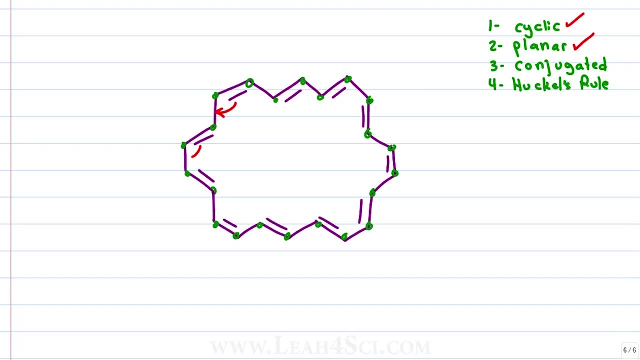 each other because there's not a single sp3 carbon to block that resonance. So we're going to use the pi bond resonance to break up the conjugation. which leaves the final question: does it follow Huckel's rule or not? Let's see. 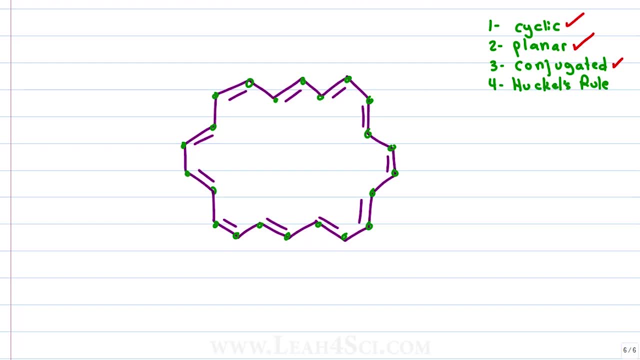 Instead of doing the math or counting the electrons, let's keep it simple by counting the number of pi bonds: 1,, 2,, 3,, 4,, 5,, 6,, 7,, 8,, 9,, 10,, 11.. 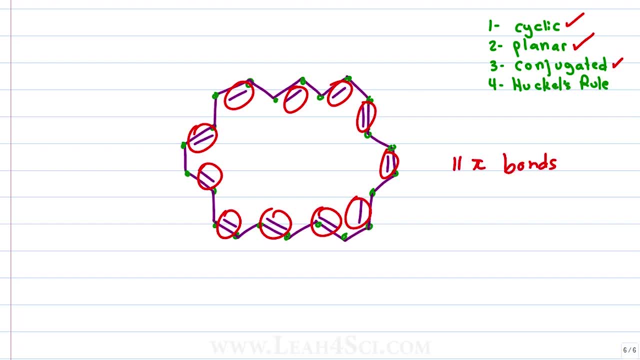 We have 11 pi bonds, or you can think of it as 11 electron pairs. An odd number of electron pairs does follow Huckel's rule. The number of pi bonds, pi or the number of electrons, depends on how many electrons follow Huckel's rule. so we want to say, yes, this is aromatic, let's prove it. but I want 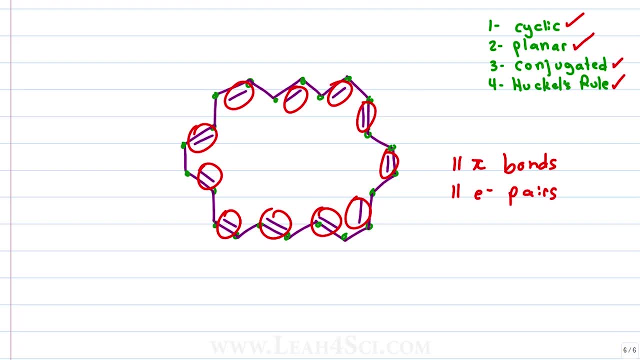 you to trust that this works so that you don't have to do it on your exam. If we did the math, we set it up as 4n plus 2 is equal to 22 electrons, 11 electron pairs, 11 high bonds means 2 per bond for 22 electrons. minus 2 on both sides gives me 4n is equal. 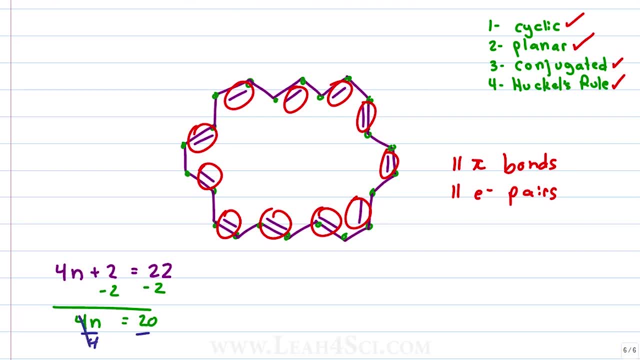 to 20, divide both sides by 4, divided by 4, n is equal to 20 over 4, which you should recognize can be reduced to 5 over 1, which is 5, we don't care that it's equal to 5,.